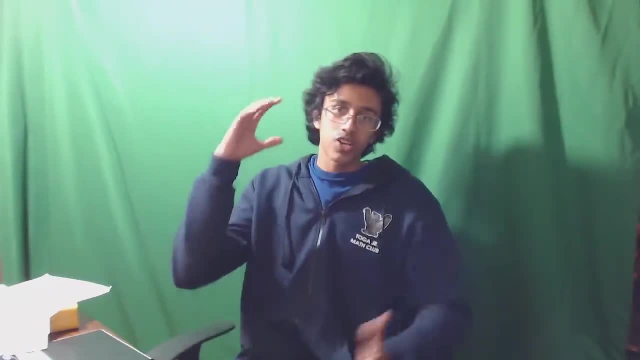 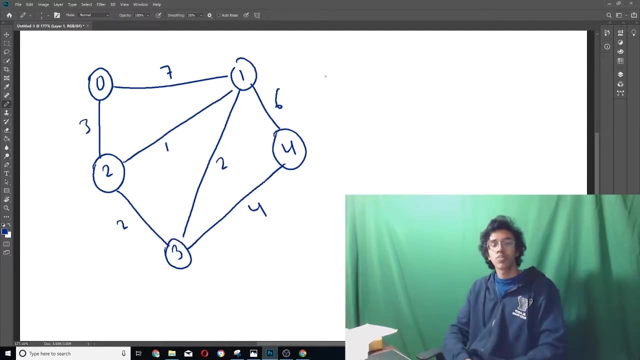 algorithm called Dijkstra's algorithm. So before we get into the actual algorithm, let's talk about what a shortest path is. All right, here's our example graph And you can probably tell what a shortest path means by the name. It's basically just a shortest path. I know Very cool, But yeah. 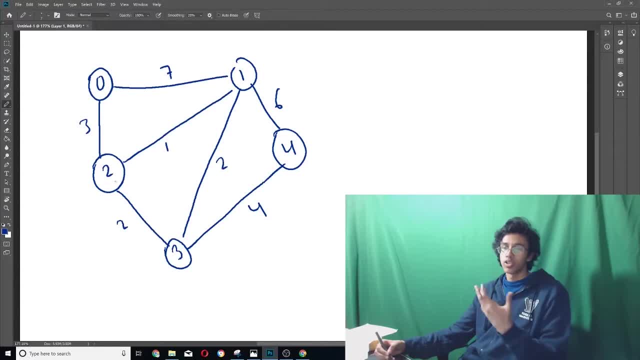 let's give an example right. So the shortest path between 0 and 2 is quite clearly 3.. And the shortest path between 0 and 1 is- no, it's not 7, because you could go 3 and then 1. That's only 4.. 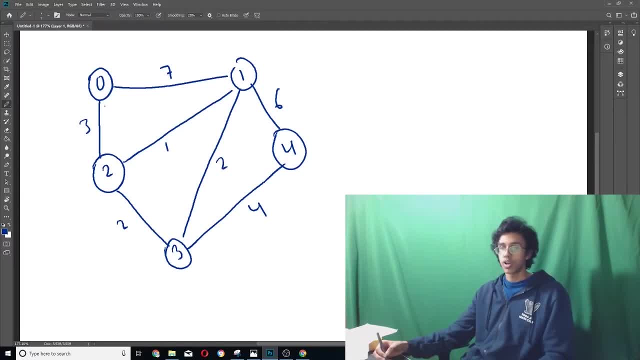 So the shortest path between 0 and 1 would be 4.. And then the shortest path between 0 and 3 would go like this, And that would be 5.. And then the shortest path from 0 to 1 would be 5.. And then: 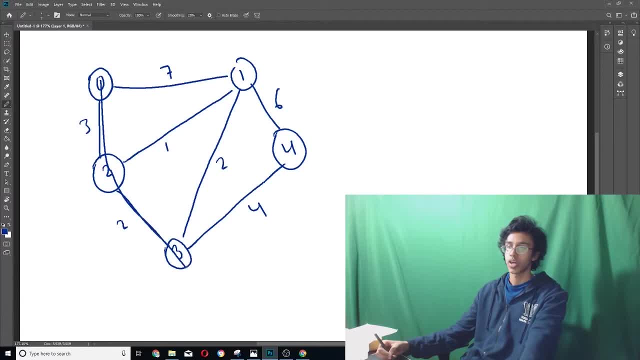 from 0 to 4 would be: you go like this, you go like that, and you go like that, And that's 9.. All right, so now that we know what a shortest path is, let's see how we actually find that. 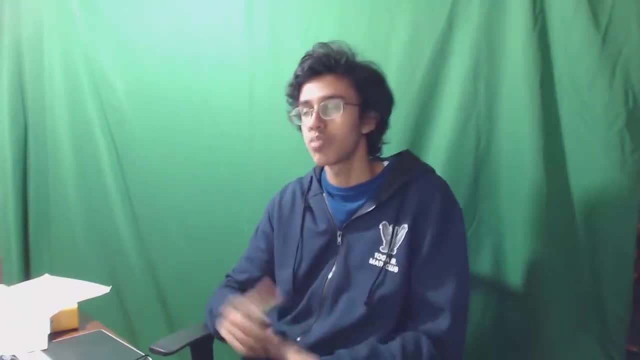 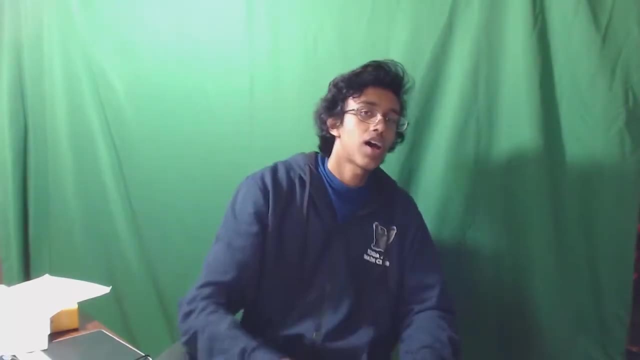 shortest path. So one dude came up with a very cool strategy. His name is Dijkstra. as you can probably tell by the name of the algorithm, It's Dijkstra's algorithm, And basically what this algorithm does is it finds all the shortest paths coming from a single vertex. So basically, 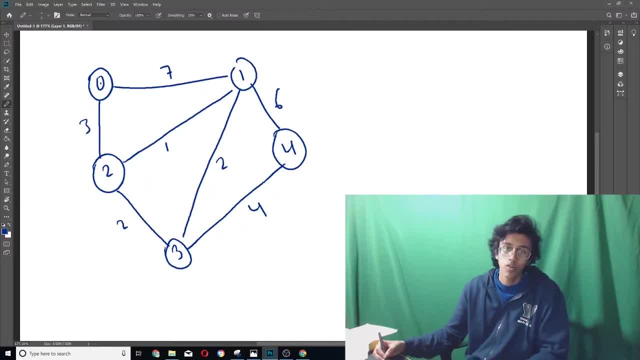 like what we just did. we were like, hey, if we start from 0, what is all the shortest paths? So we found 1 is 4.. We found that 2 is 3.. We found that 3 is 5.. 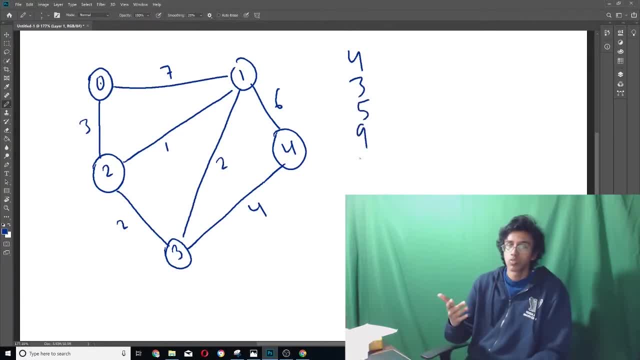 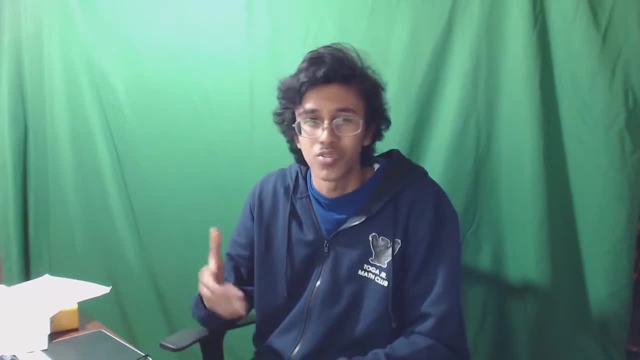 And we found that the shortest path to 4 is 9.. So, basically, what Dijkstra's would do is give you this list- Well, and of course 0 is 0 from itself, so it'd also give us that. But if your algorithm can't do that without the help of Dijkstra's, that's kind of sad. 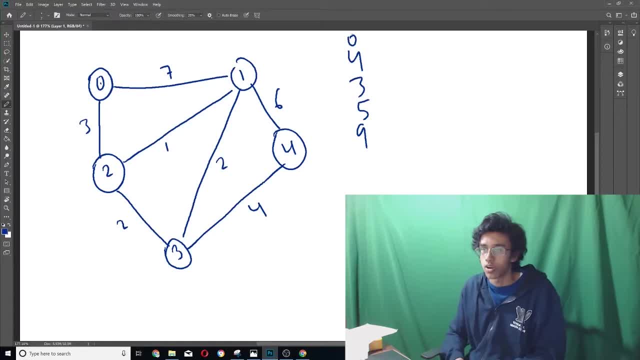 not gonna lie. So how does this epic algorithm work? So, basically, what it does is it starts from your starting vertex at 0.. And then it's like the distance from 0 to 0 is 0, so it has like a grid of distances. 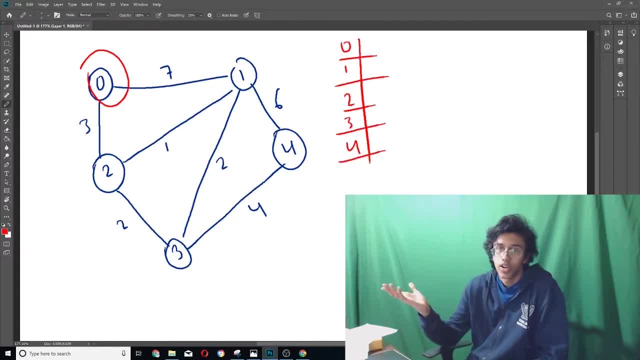 And this grid of distances starts out empty, because we don't know any of the distances, except at the very beginning. we look at 0, and we say, hey, how far is it from 0?? We know it's 0,, so we just put 0 over there. 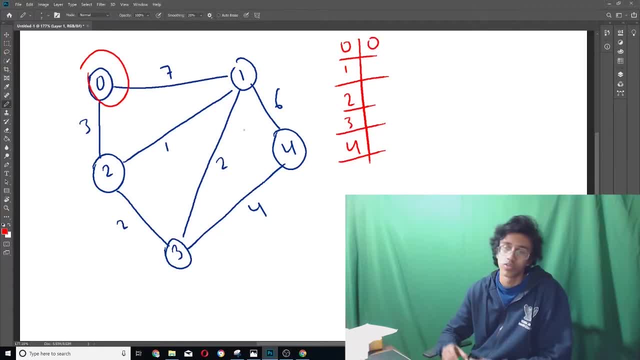 But we don't know what any of the other things are, so we don't change them yet. But then what we do is we go from 0, and we look at its neighbors. So first we look at 1, it's 7 away from 0.. 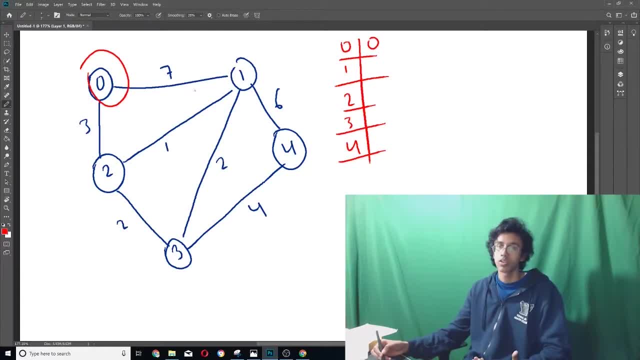 So the closest path we've found to 1, the shortest path to 1, so far, is 7.. So we'd write a 7 in here and then we circle that one and then move on to the next neighbor, which is 2.. 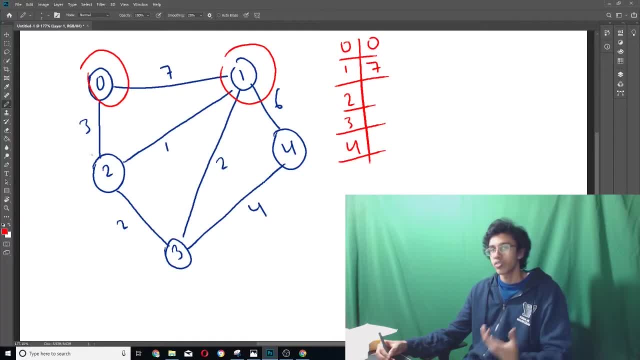 So we go to 2,. we'd say our shortest path that we've found to 2 so far is 3.. And then we circle that boy And then, once we look at all of its neighbors, we go back to 0, and we're like 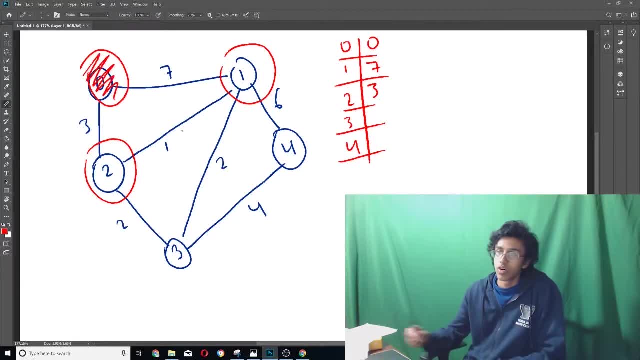 we're done with that, so we don't need you anymore. so we cross it out All right. now, instead of taking things in the order that we looked at them, we take them in the order of how close they are to 0.. 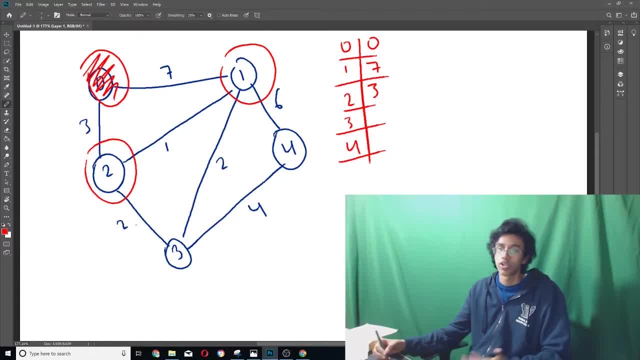 So if we look at the two things that we still have circled- 1 and 2, which one is closer to 0? We see that the answer is just 2.. So we would look at 2 next, And then we're like: what is the neighbors? 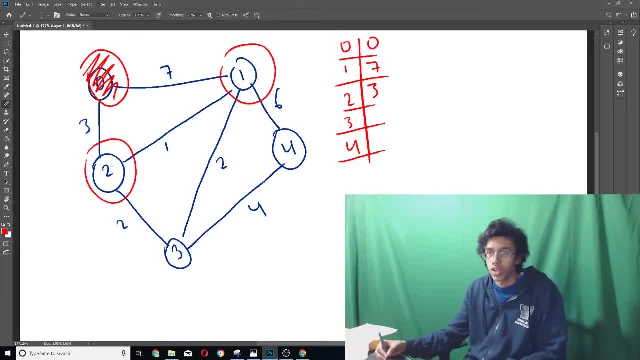 So we first look at 0, but we already crossed it out so we don't have to worry about that. We look at 1.. Well, the distance, total distance from 1 to 0 would just be the distance to 2,. 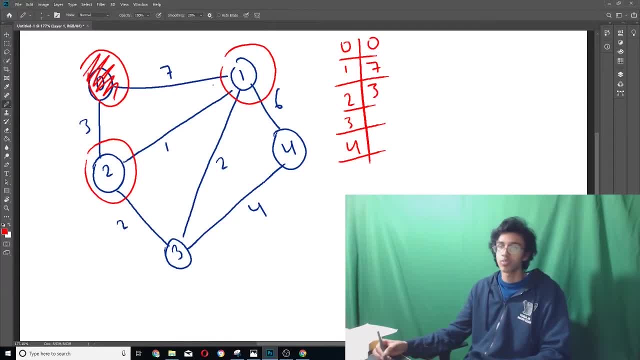 plus the distance from 2 to 1.. So it'd be 3 plus 1.. So it'll be 3 plus 1 is just equal to 4.. 4 is less than what we thought our shortest path was for 1.. 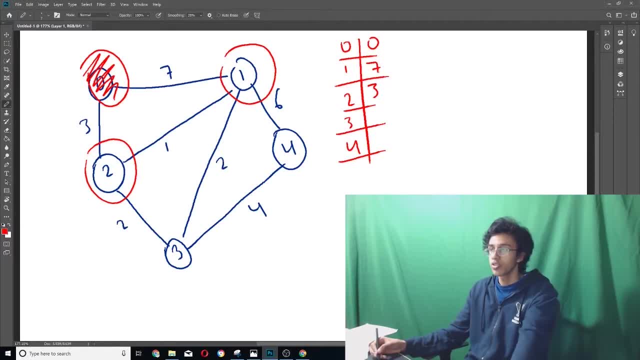 We thought it was 7. But that's not right. So what we do is we just change this over here to 4.. Then we look at the next neighbor, which is 3.. And then we're like: OK, so 3,. what is the total distance from 3 to 0?? 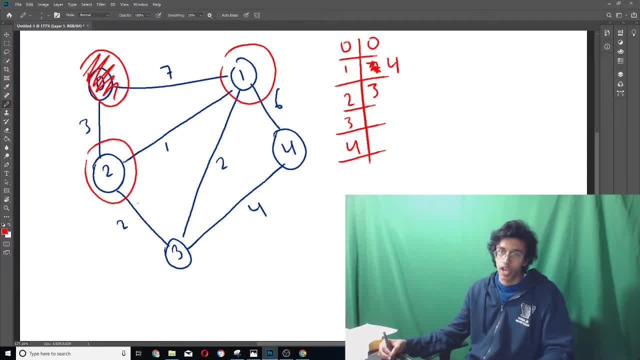 It's just the distance from 0 to 2, which we know is 3.. And then we add in this edge over here, which is 2.. So our total distance would just be 5.. So we're like, hey, the shortest path we've found in 3 so far is 5.. 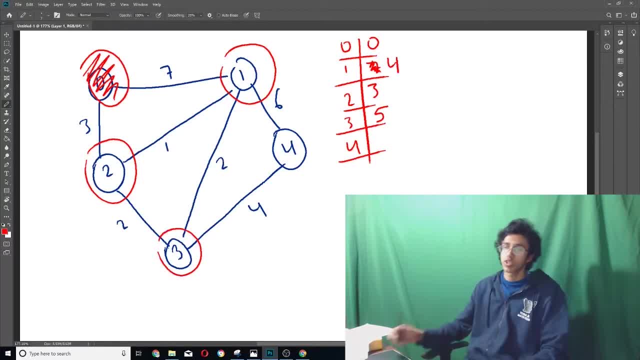 And then we circle that And cool, we looked at all the neighbors of 2.. So we just cross it out. All right, epic, Two down, three more to go. And now which one do we look at? We've got to look at 4.. 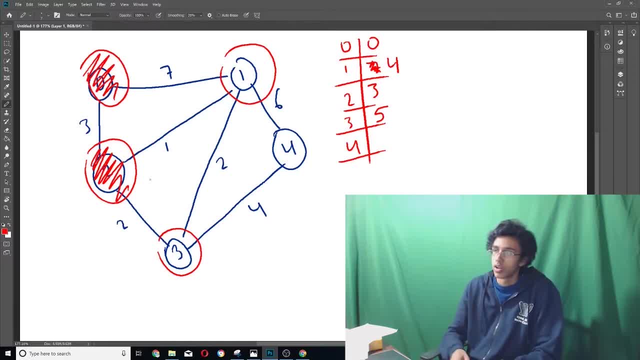 We've got to look at 1.. We've got to look at 3.. Which one is closer to 0?? And we look at our numbers over here in this little data table thingy. We look at 1,, 4.. 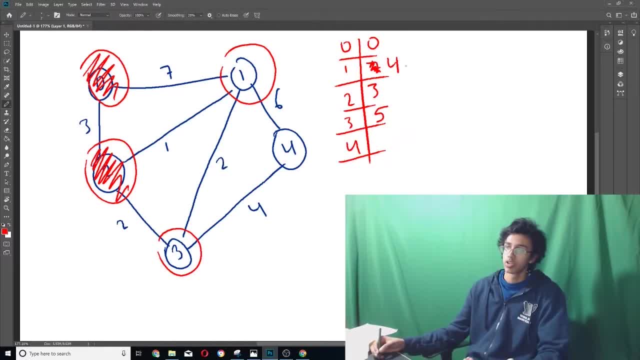 3 is 5.. And we're like the shorter one is just 1.. So we look at 1 first. Look, the neighbor is 0.. Nope crossed out 2.. Nope crossed out 3. 3,, however, is kind of interesting because we could get from 1 to 3, right. 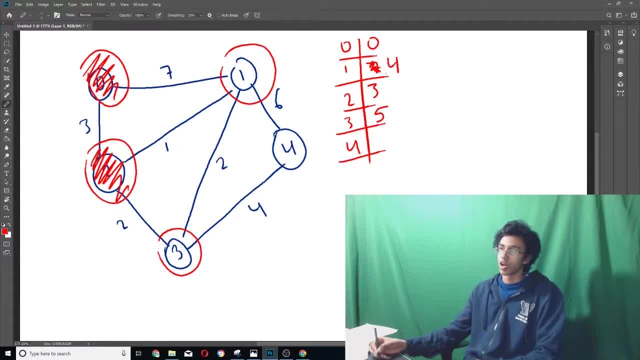 So the distance from 1 to 0, we know, is 4,, as we have over here, And then the distance from 1 to 3 is 2.. So the shortest path to 3, which goes through 1, would be 6.. 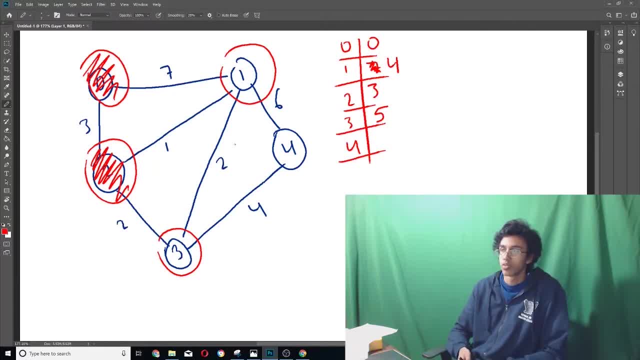 But we already found a better version of it, So we don't change anything. We already know that the shortest path to 3 that we found so far is 5. So there's no reason to change it to 6.. Why would you want to take a longer path to find the shorter path? 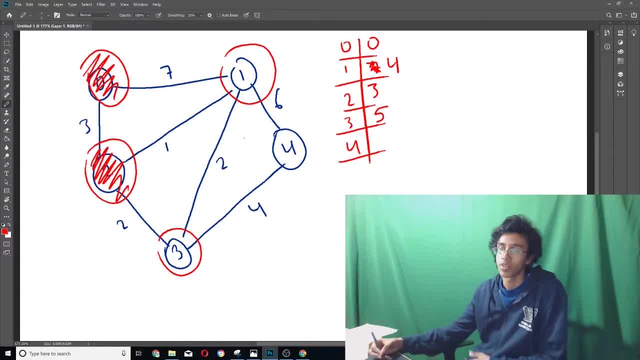 That doesn't make any sense. All right, so then we're done with 3.. Now we have to look at 4.. All right, so basically the distance from 0 to 1 is 4. And then we add in the 6.. 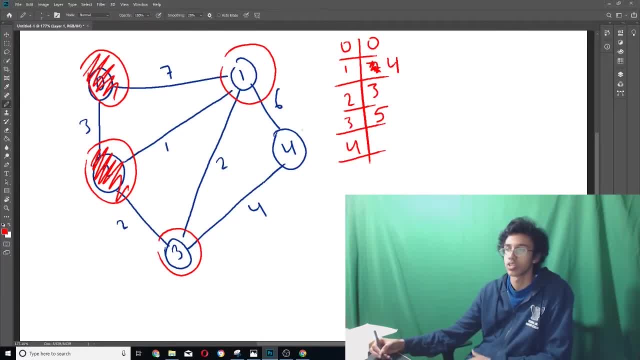 And then the distance from 4 to 0, our best, shortest path so far is 10.. So we put 10 and we circle it. Now we're done with 1.. Move on to 3.. We look at its neighbors. 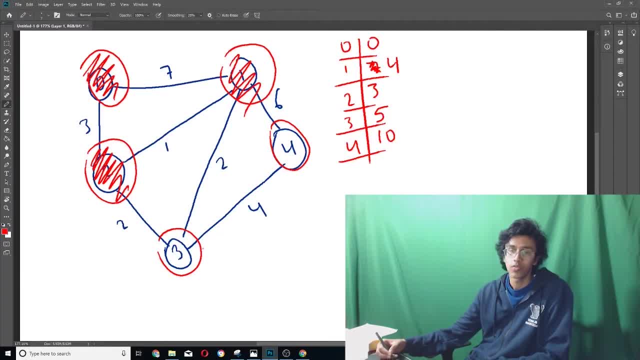 All of this are crossed out except for 4.. And then we do 5,, which is the distance from 3 to 0,, as in our table, And then we add 4 and we get 9.. And 9 is better than 10, so we cross that out. 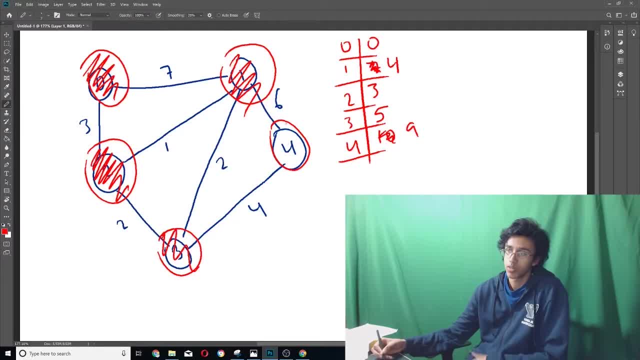 Set it at 9, cross this out, And then 4 can't have any neighbors, so we cross that out. Cool, Wait a minute, Wait a minute. This is exactly the list that we found at the very beginning of this video. 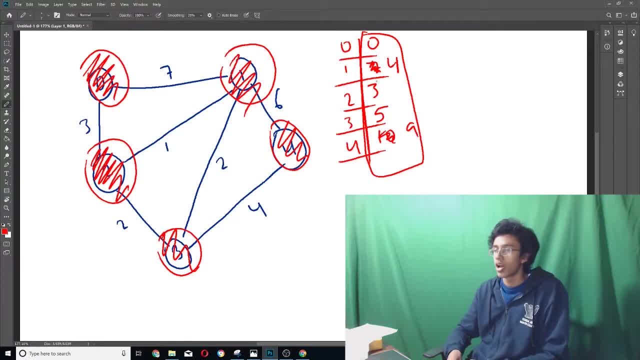 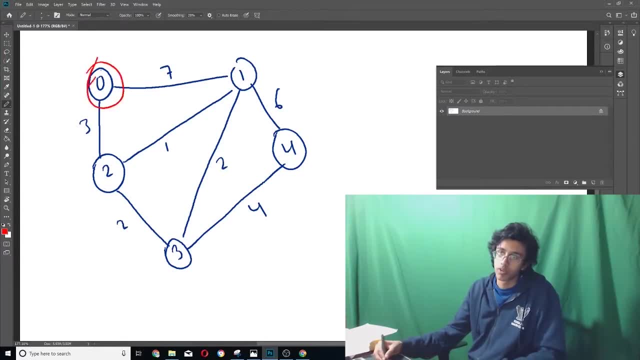 It's all the shortest paths from the vertexes to 0.. How did we do that? It's actually crazy. So the intuition basically goes like this: Let's say that we're at the stage where we've crossed out 0 and 2.. 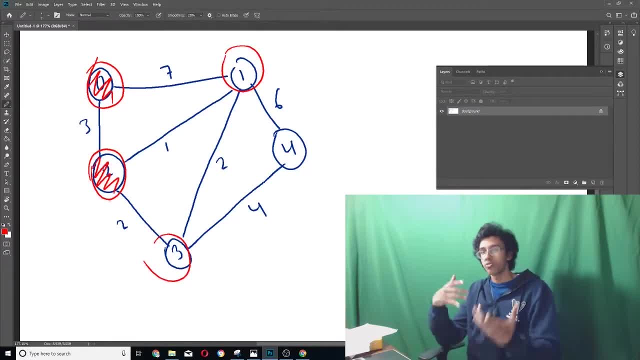 And we're looking at either 1 or 3.. So now should we look at 1 or 3?? That is the question. So basically, at this stage, we've basically looked at all the shortest paths that go through 0 and 2.. 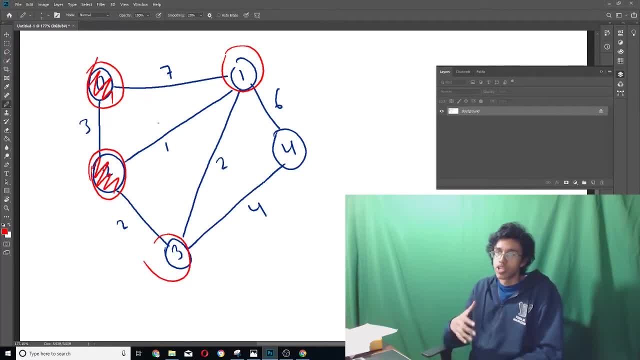 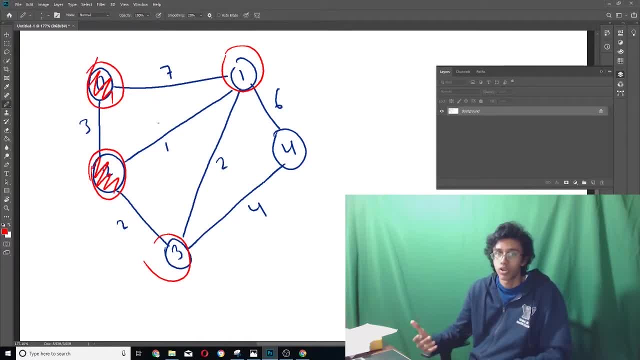 And if the distance from 1 to 3 was something less than 1,, then a shortest path through 1 would be better. However, can a shortest path to 1 go through 3?? No, because the shortest path from 0 to 3 is 5.. 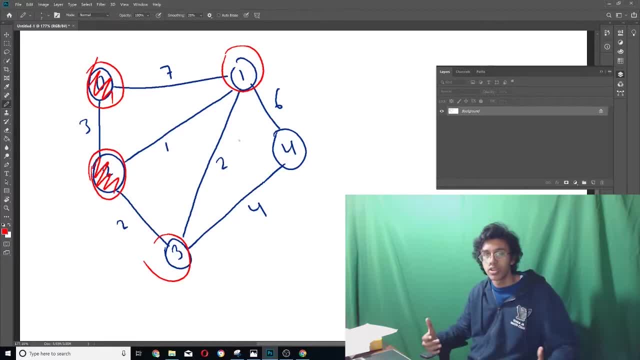 So any shortest path going from 0 to 1 that goes through 3 would have to be at least 5.. But we already have the shortest path we found so far as 4.. So it doesn't even make sense to look at 3 first. 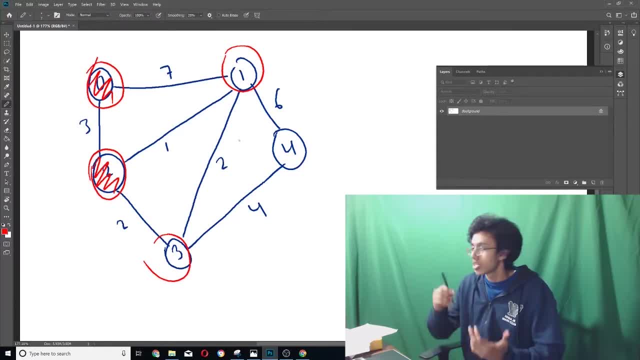 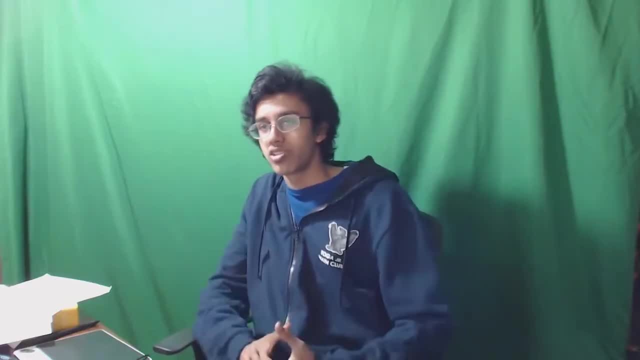 That's why we look at 1 first, Because it's guaranteed to not go through any of the other points we're considering, And that's how we find the shortest path. You don't really have to know exactly how directions work, but you basically just have to know that you have to look at. 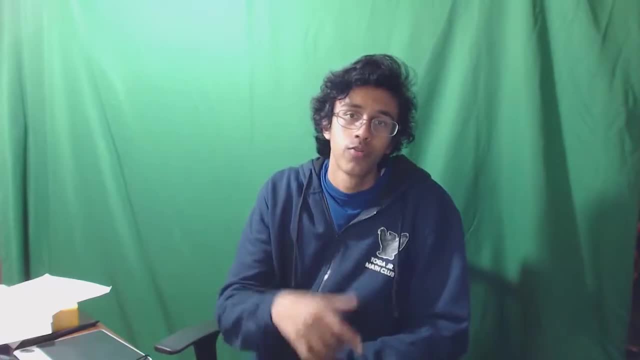 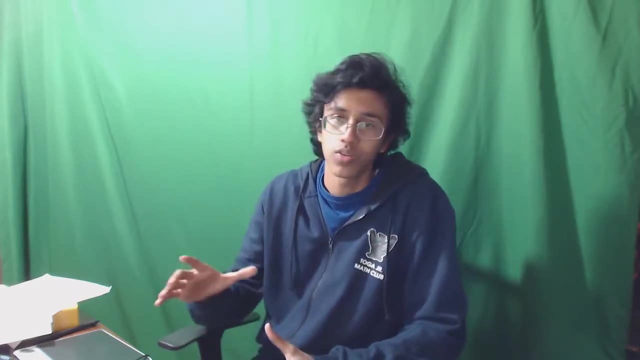 vertexes that are vertices that are closer to 0 first. So the way we would do this in code is using something called a priority queue. So basically, what a priority queue does is it spits out the smallest number or the biggest number, depending on how you do it. 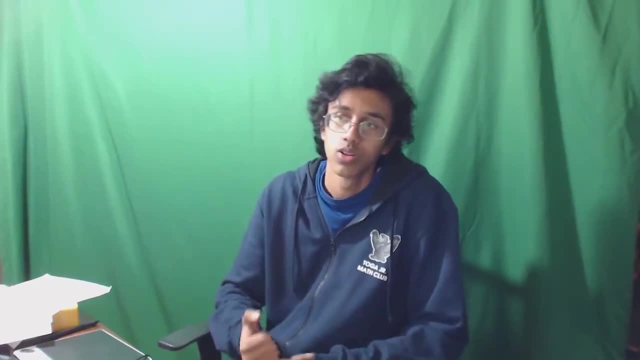 And that's good, because we want to spin out the smallest number and then look at that number and look at all its neighbors. So let me show you the code, Alrighty? so this is how it starts off. So we have n vertices. 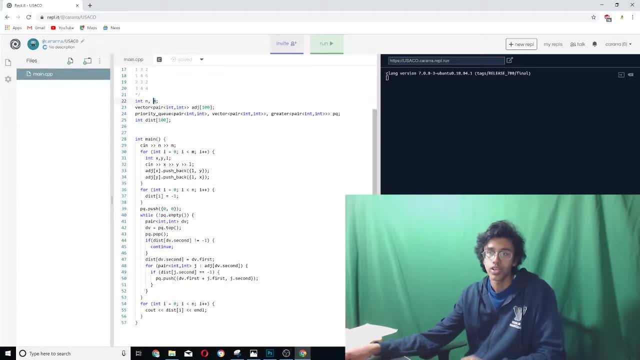 And m edges And then basically this is our adjacency list. And then this long line of code is basically how you make a min priority queue. So by default in C++ our priority queue orders it from greatest to least, But we want to spin out the smallest first. 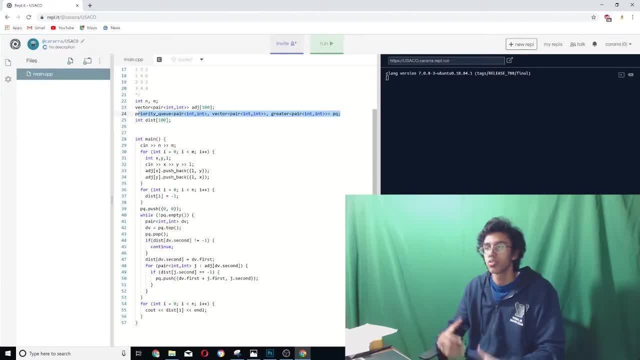 Because we want to look at closer vertices first. So we basically have to do the reverse. So, in order to make it reverse, you basically have to do this whole thing over here And then add the greater thing over here, And then, over here, we have our distance. 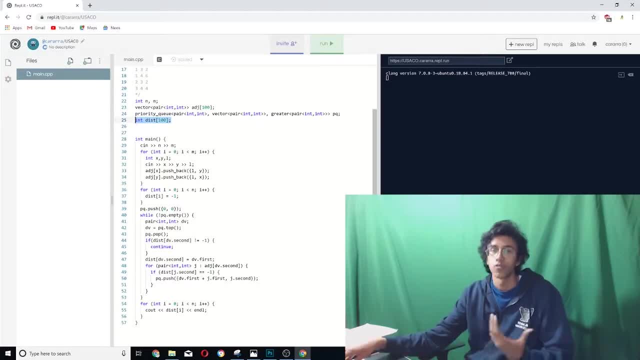 Array that you could see by our data table in our example. So first we read in our n and our m, Then we read in all the edges, which are composed of the starting vertex, the ending vertex and the length, And then we put it in both x and y in our adjacency list, because the edges are bidirectional. 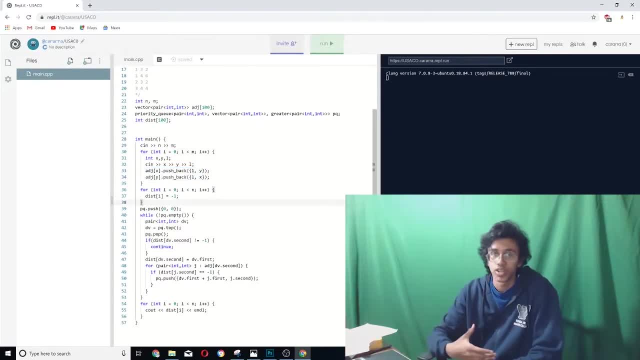 Then we set all our distances to negative one, which basically means that they're not set yet, And then we put our zero- zero into our priority queue, Which is basically like our circling, the zero- zero in our example- And then, while we have more vertices, we're going to put our zero- zero into our priority queue. 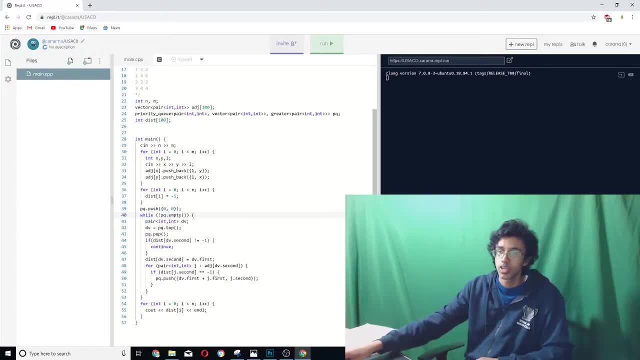 And then, while we have more vertices at a circle that we haven't looked at yet, we basically look at the first one and if it's already been looked at and crossed off and everything, then we don't look at it. But if it's not been crossed off, then we set its distance to the best distance we found. 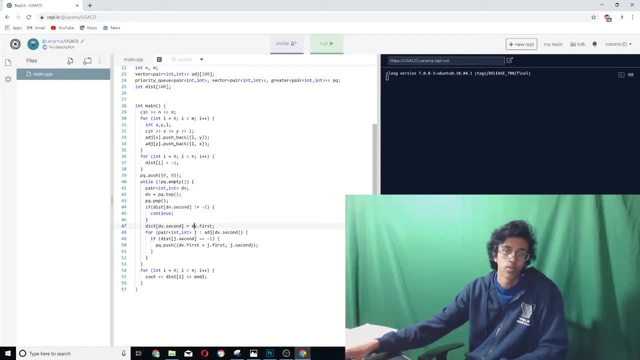 Then we look through all its neighbors and then push them with their lengths to the priority queue. So this is kind of confusing a little bit because I use a lot of pairs. So the reason why I use pairs is because you can match a length to a vertex. 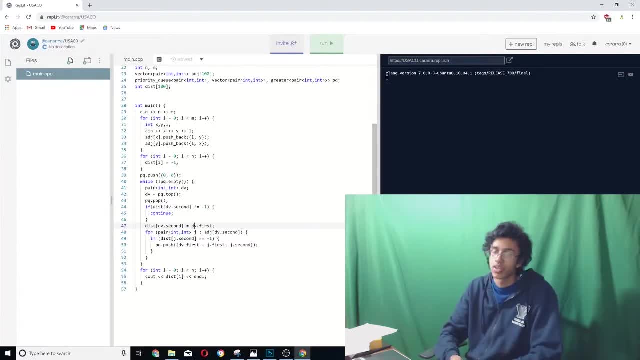 So basically in our adjacency list it has an end vertex and its length And then in our priority queue we put in the distance from the vertex to the zero and the actual vertex itself. So for example, if we wanted to say one is like eight away from zero, 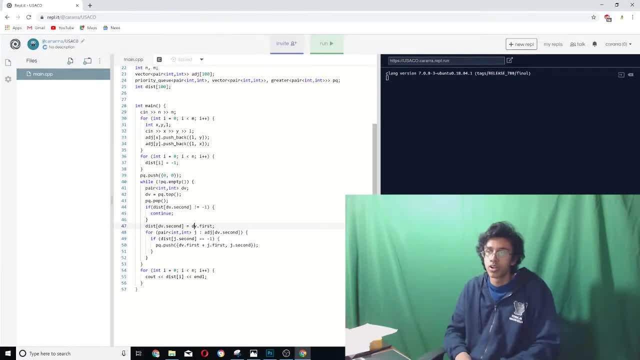 then we put eight comma one in our priority queue And because we're trying to minimize it, it'll check: is eight the smallest one? And if eight is the smallest thing, it'll print that out. And then, at the very end, what we do is we just print out all our distances. 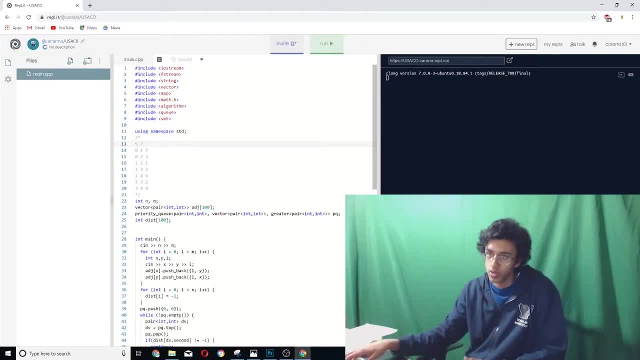 So right here is how Yusuko would represent the graph we used in the example. Let me put it in: This is an algorithm, real quick, And we get exactly what we expected: 0,, 4,, 3,, 5,, 9.. 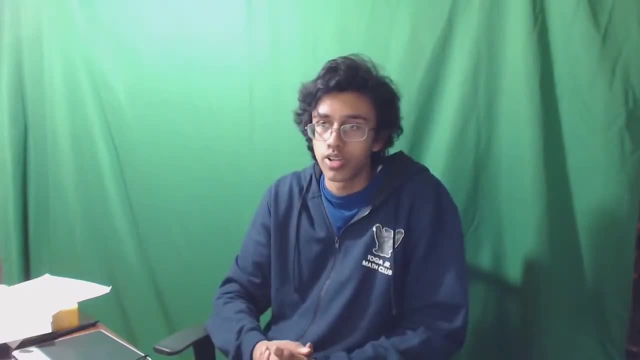 The magic number. All right, so that's basically all you got to know for Dijkstra. If you want to learn exactly how to code it, just look at the code that I showed in the video and try to like memorize how the structure works. 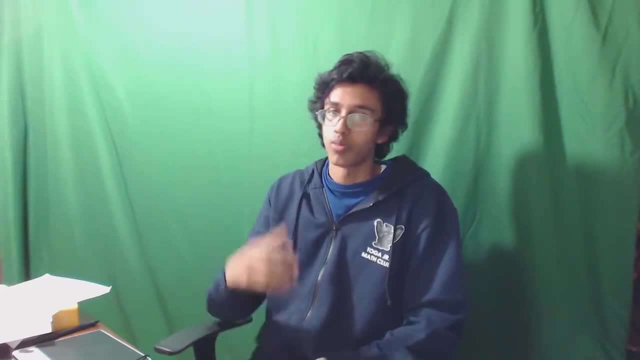 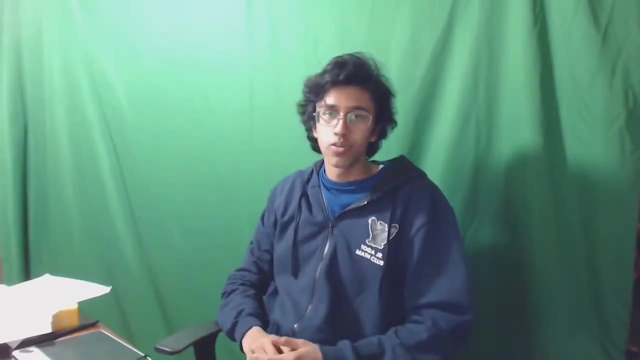 The reason why Dijkstra is so useful is that you could find in a pretty fast time n squared. to be specific, you could find the distance between any one point and any of the other points. So Yusuko usually gives us in two ways. 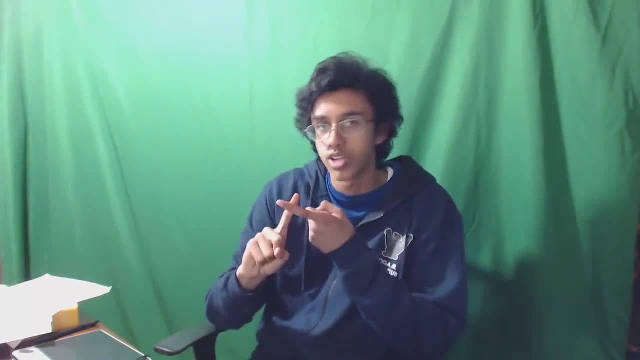 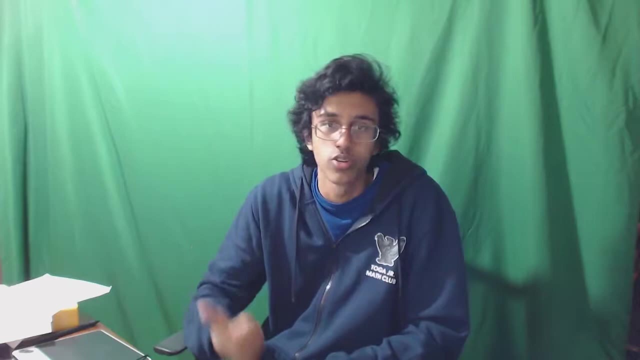 Either they say: find the place that's closest to a certain destination or find the destination that's closest to a certain place. So if Bessie starts from this field, which field is closest to her? Or if she starts from this field, how long will it take her to get to this field over here? 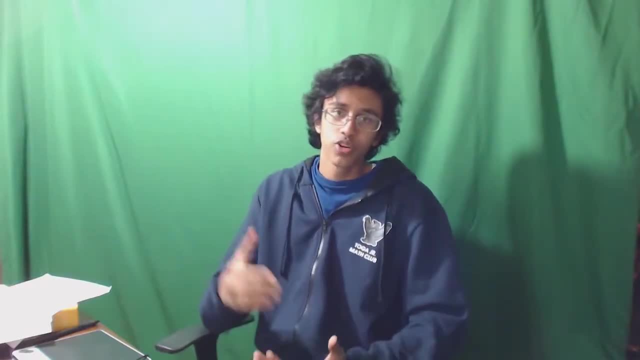 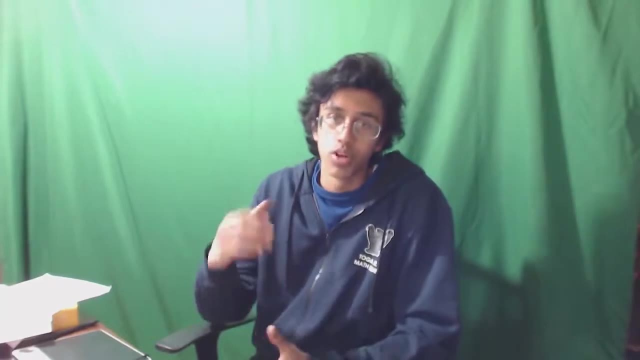 So yeah, that's all I got to say about Dijkstra. It's actually a super useful algorithm, One of like the first algorithms I learned after DFS and BFS, And it's actually kind of cool once you understand it. It's really similar to Prim's algorithm as well, if you've heard of that. 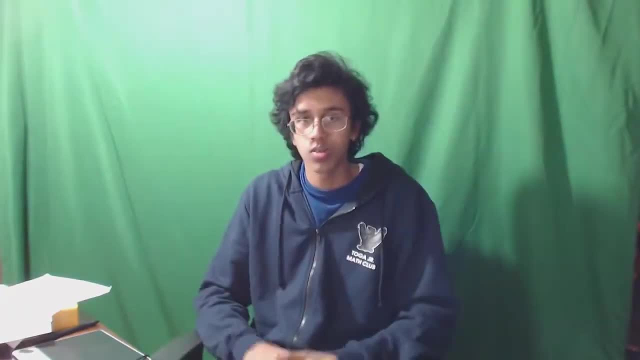 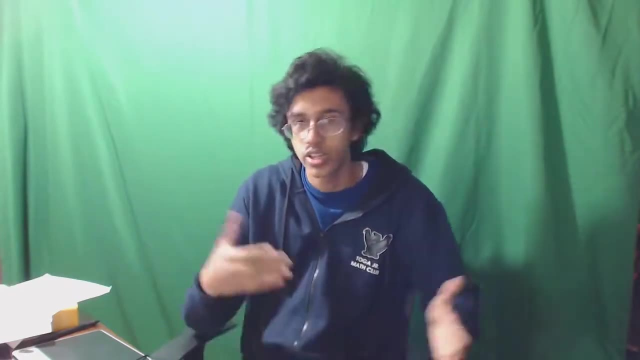 And I'll probably explain that in a future video, So stay tuned. Alrighty, thank you guys. so much for watching. As always, we'll be back next time. If you enjoyed the video, leave a like and subscribe for more. Comment down below if there's any specific musical crash courses or any like. 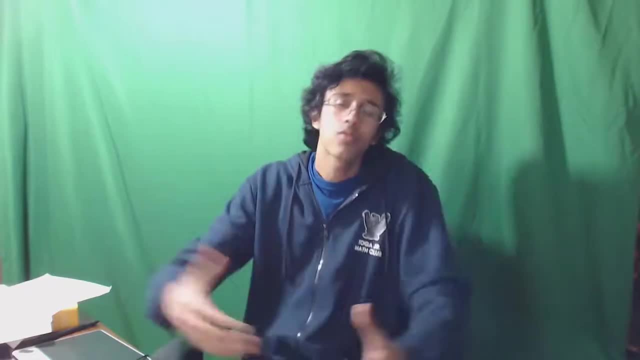 algorithms you want me to cover And other than that. thank you guys so much for watching and see you guys next time.